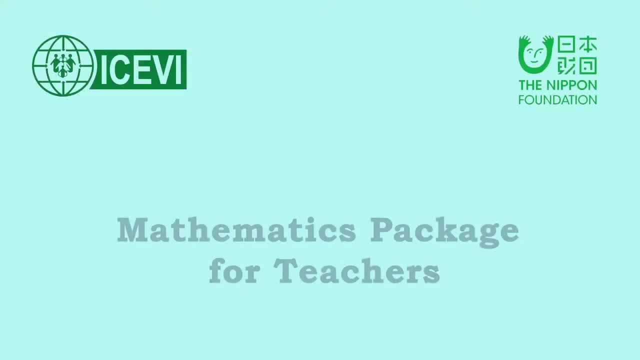 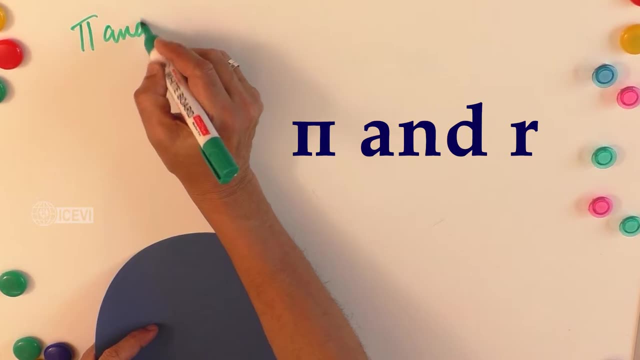 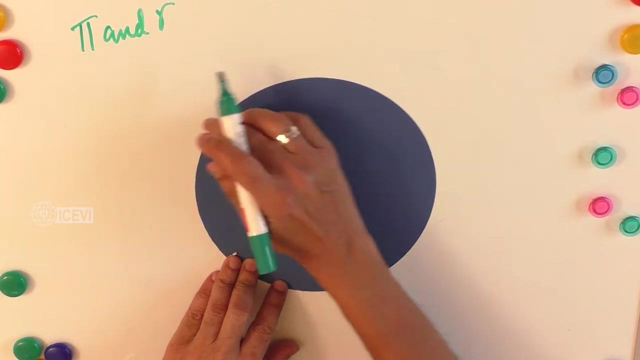 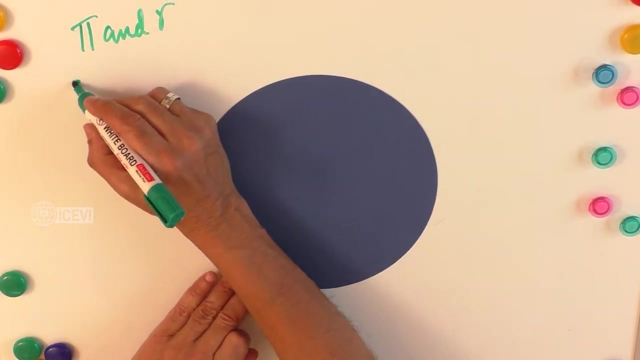 The ICBI, the Nippon Foundation Mathematics Package for Teachers. Title of the video: Pi and R. In using circle we always refer to the pi and r. So when we take a circle to find out the circumference, we use the formula 2 pi- r. 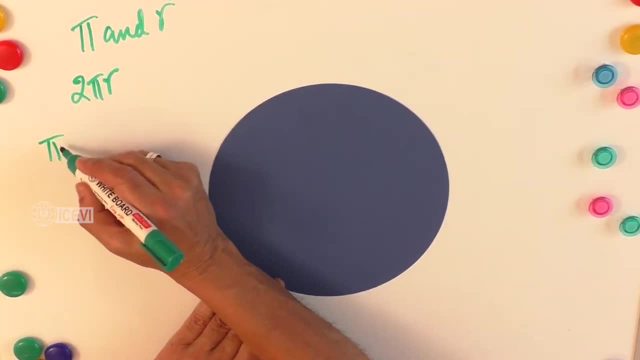 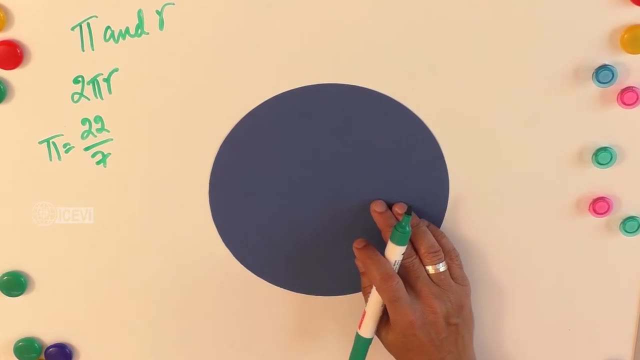 And we always say that pi is a constant, that is, 22 by 7. And we use this to calculate the circumference of the circle. There is a relationship between pi and r And the child can be given this practical experience of linking the pi and r. 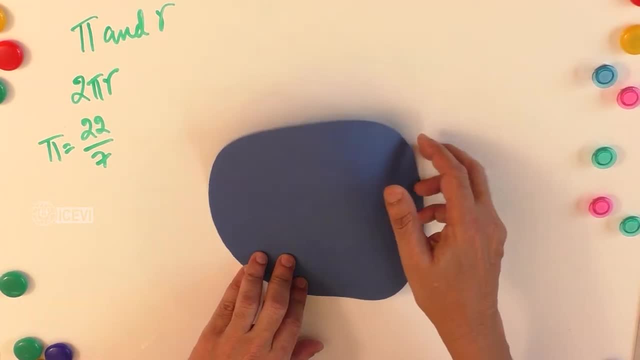 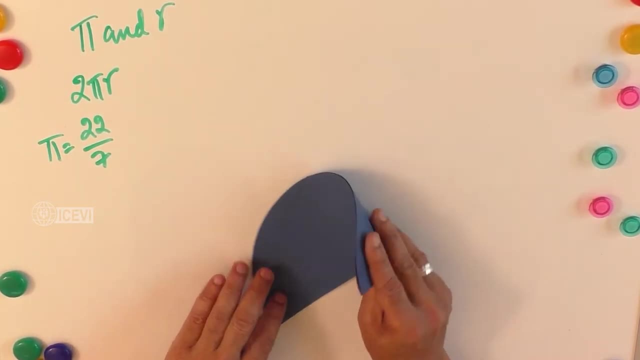 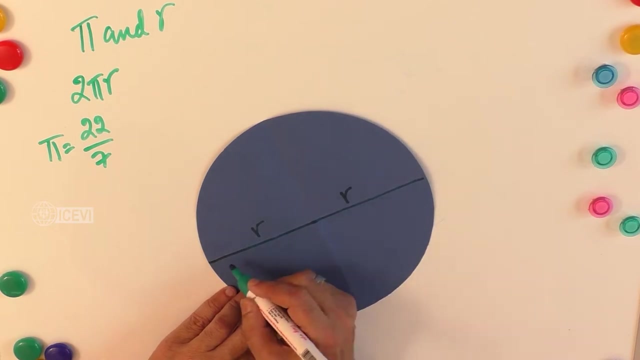 Now let us take a circle And then fold the circle To get a diameter, And then we fold it again vertically To get the radius. Now what is the relationship between the diameter and the radius? The diameter of the circle is 2 times of the radius. 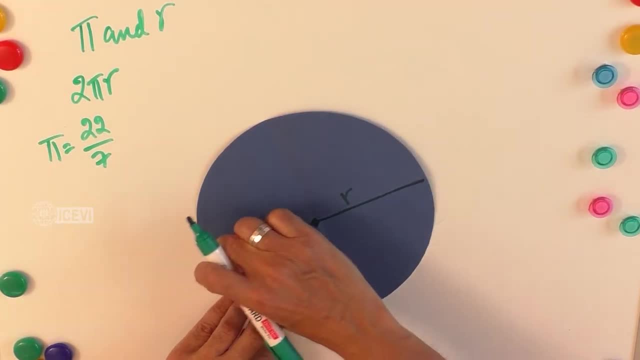 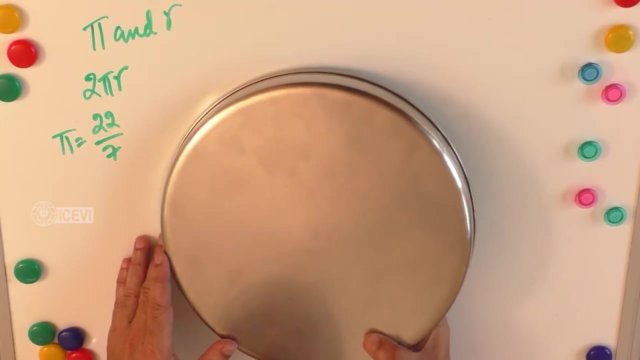 Now, the diameter and the circumference of the circle Are linked in certain proportion. So let us find out that, using real objects And giving practical experience to the child. Now let us take a plate. Let us take a plate And let us find out the circumference of this. 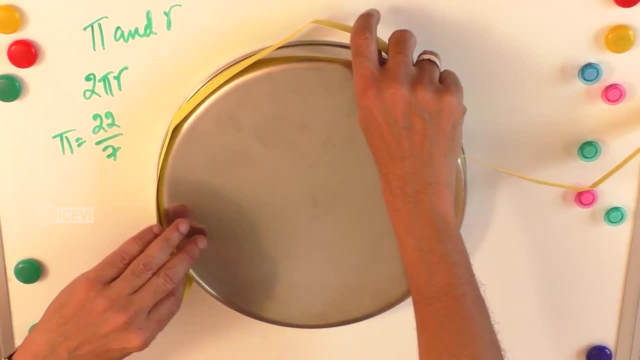 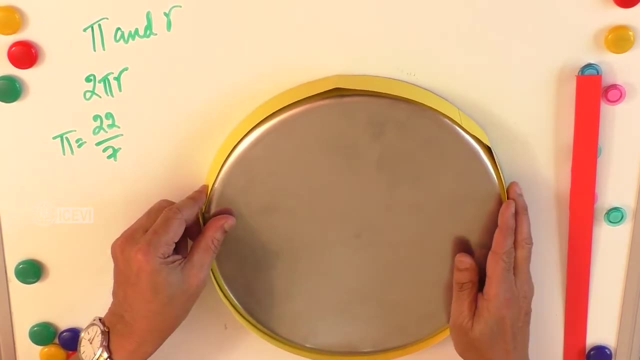 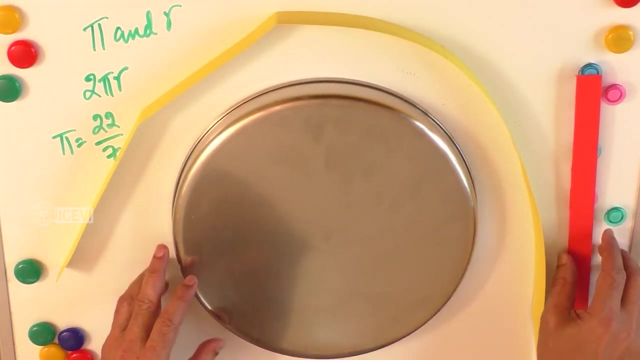 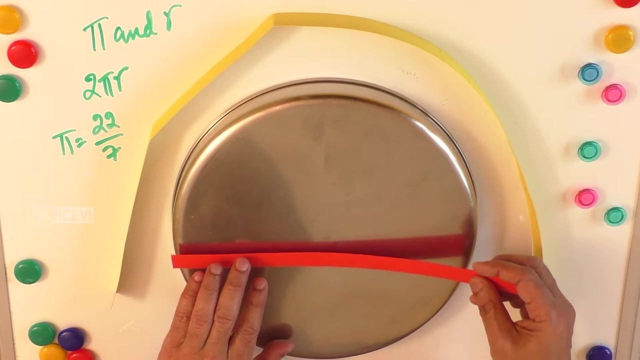 Let us find out the circumference of this Using a paper strip. Right, We have used this paper strip to find out the exact the circumference of the plate. Now we have to find out the radius, or the diameter. Now, in a plate like this, it is easy to find the diameter than the radius. 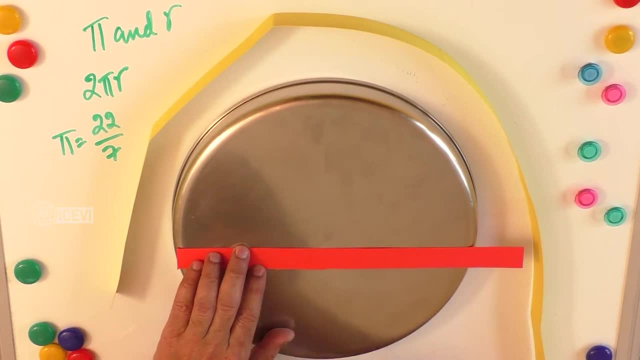 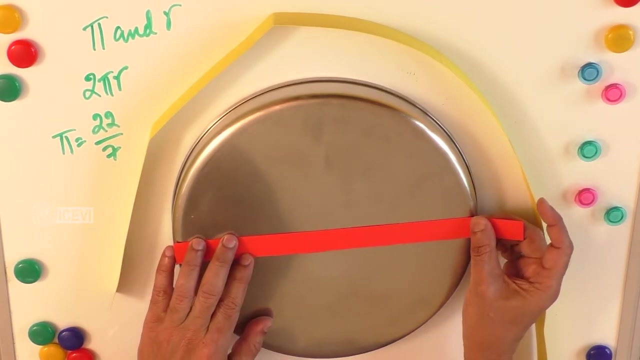 Because it is very difficult to find out the center of this plate. Now have an approximation of the radius, The upper half and the lower half, And then try to find out the diameter of this plate. So approximately I find a diameter of the plate using this paper strip. 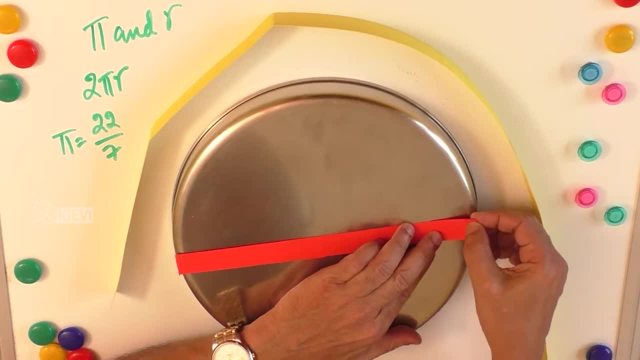 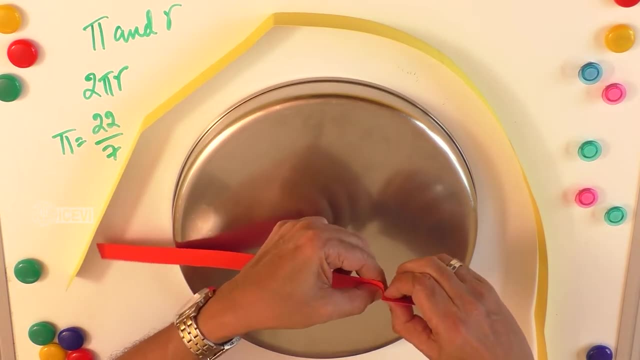 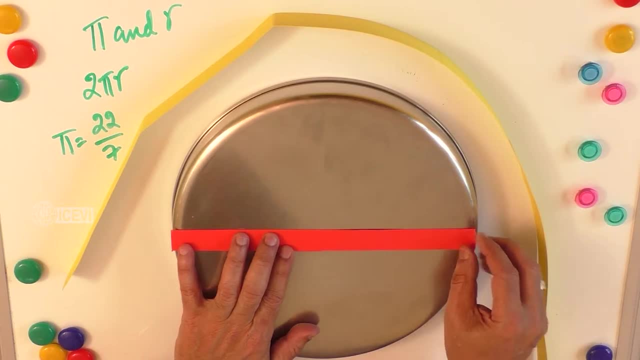 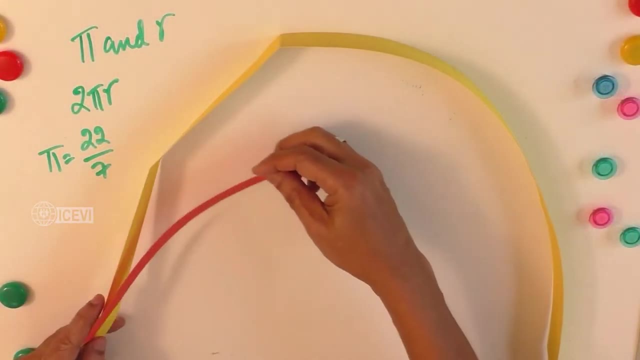 Now I have made a paper strip which is the diameter of this plate. Well, it may not be exact, You know. approximate measurement is OK. Now let us find out the relationship between the the circumference of this plate and the diameter. 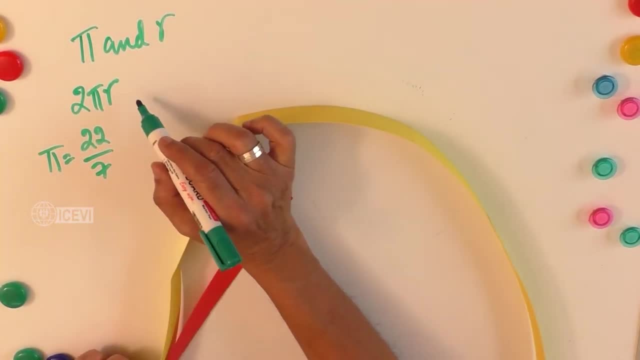 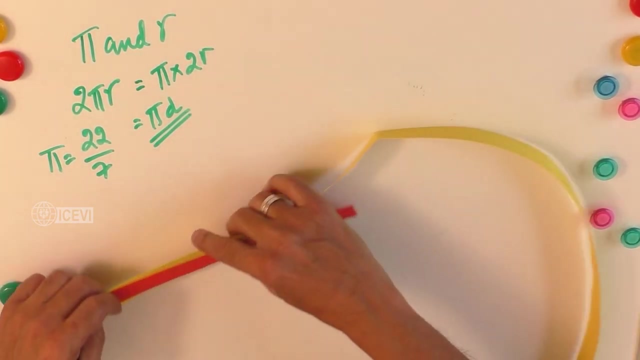 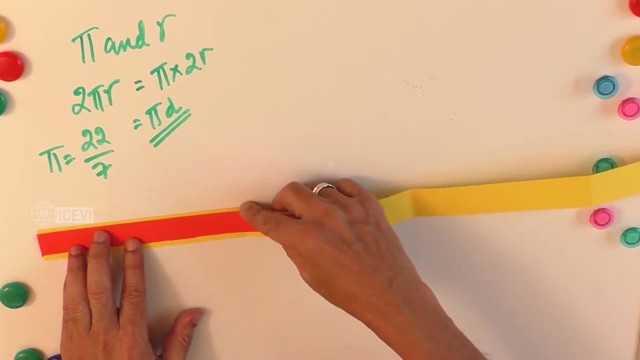 So when you see two by R, two by R is nothing but Pi into two R, That is pi D. Okay, so that is diameter. now let us find out how many times of the diameter we get in the Circumference. this is one, and. 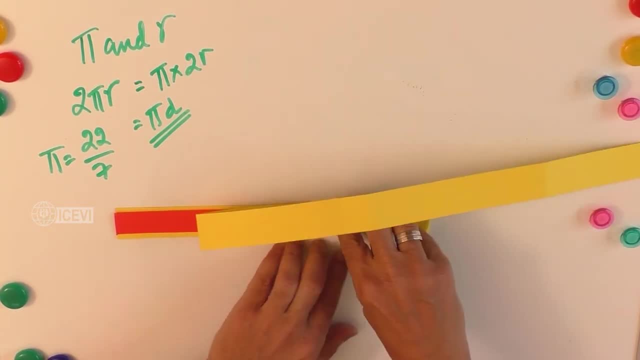 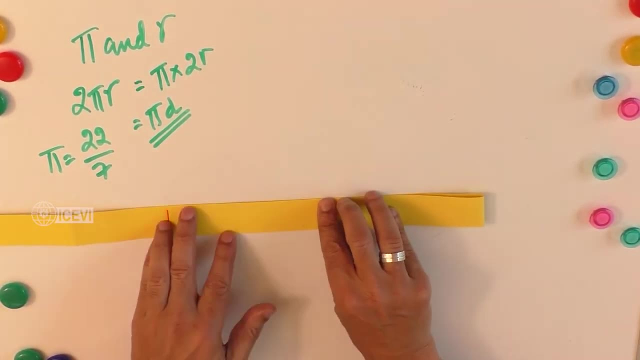 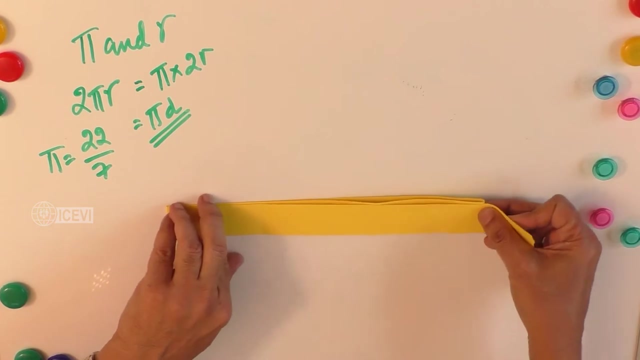 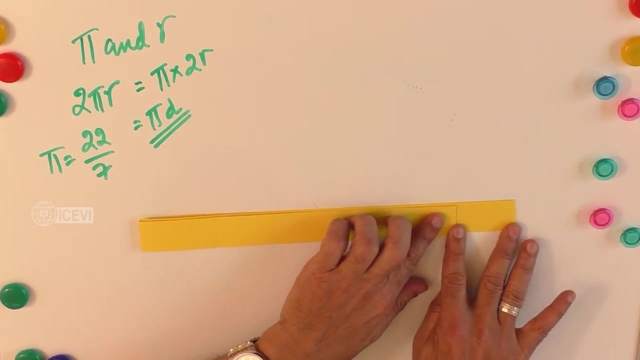 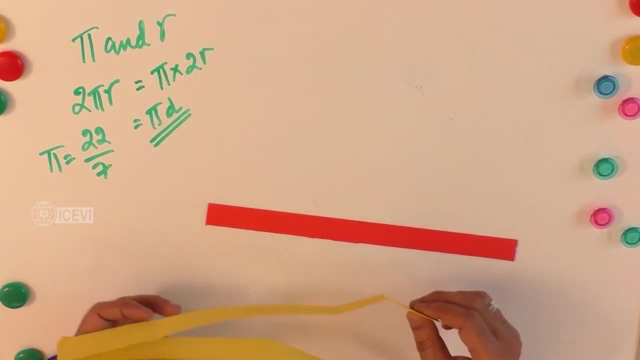 you can simply fold that paper and Two right, and then you can turn it and then Make one more time. So, three right, so and, and a portion left. Well, this is nothing but the 1, 7th of the portion. So what happens? you know, the diameter is linked to the pie in such a way that 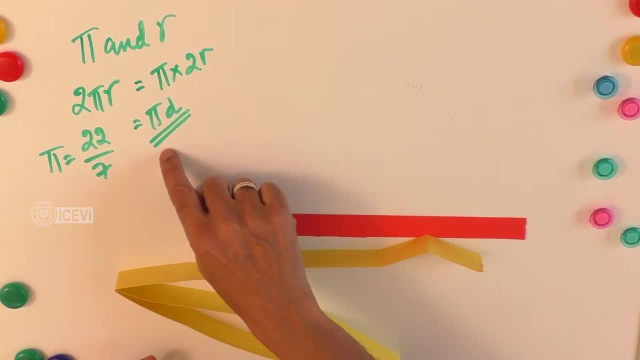 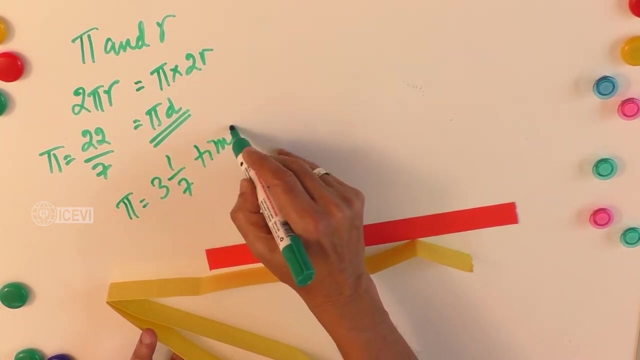 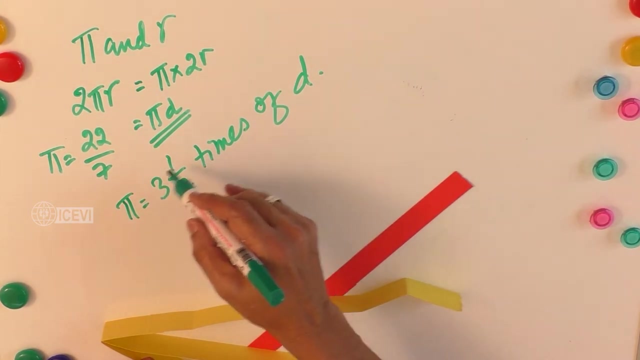 the pie is 3: 1 by 7th time of the diameter, the diameter the pie is. the pie is approximately 3, 1 by 7th times of The D. so that means the circumference. when you have the diameter, the circumference is pi D. 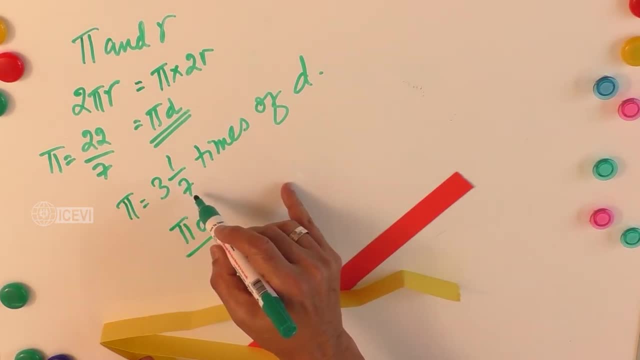 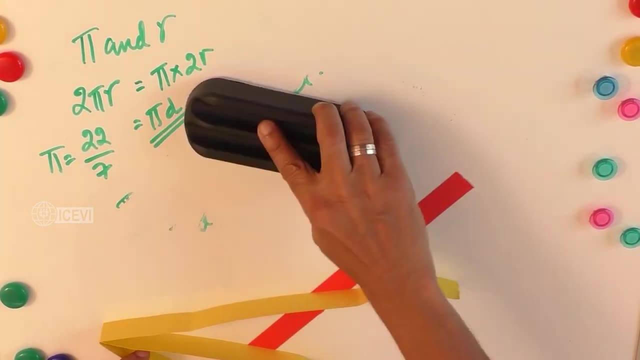 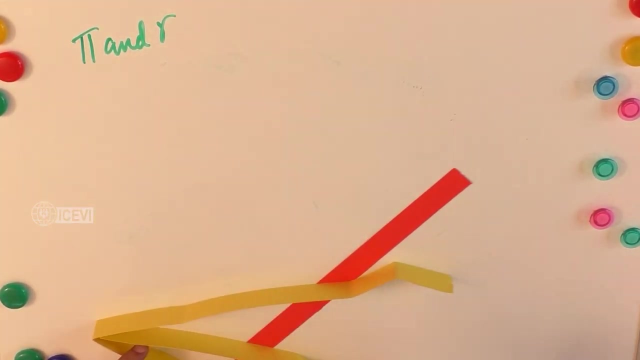 so that is, pi is 3, 1, 7th times of the diameter. Let us prove this with another example to. we have used a big plate. now Let us take a small lid and see you know how we get this measurement. now Let us take a small lid.